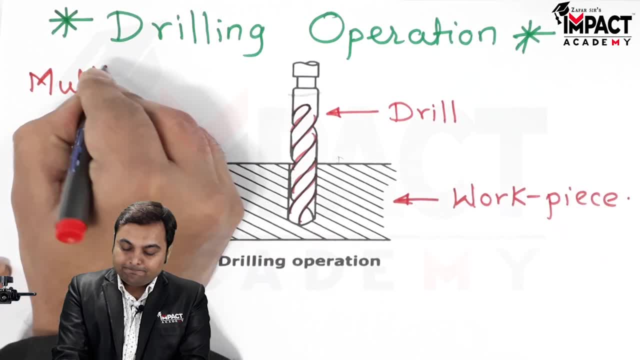 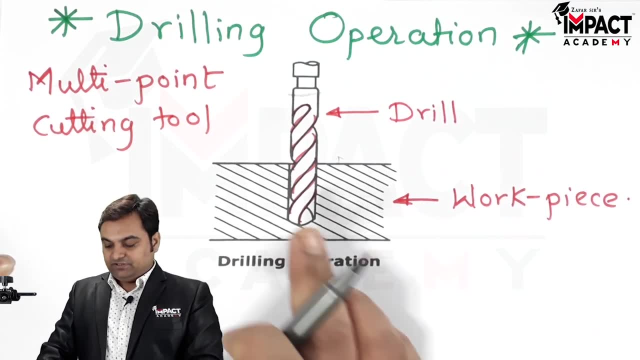 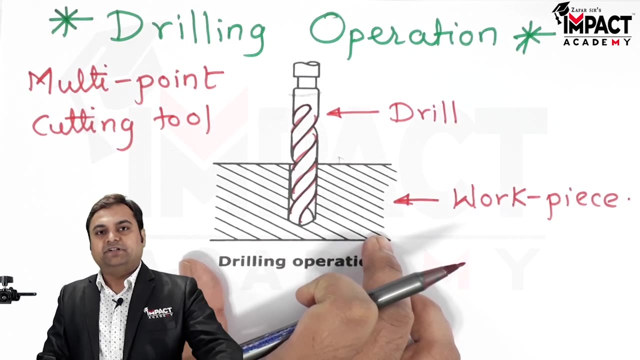 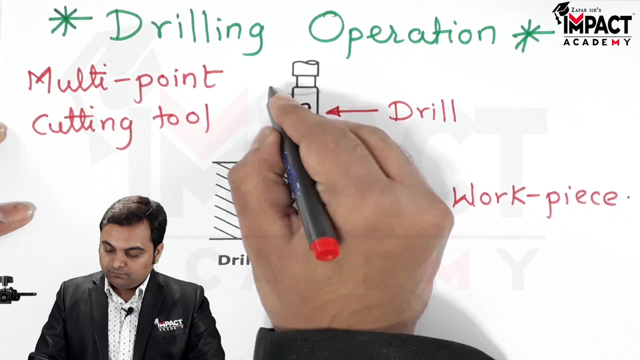 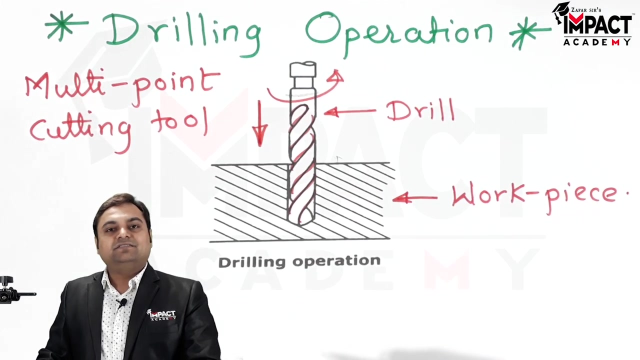 as a multi-point cutting tool and this drilling operation is performed in such a way like the workpiece. If it is performed on a drilling machine, then the workpiece is kept stationary, the drill is rotated. The drill is rotated. at the same time it is fed inside the workpiece. So that is done in case of either portable drilling machines. 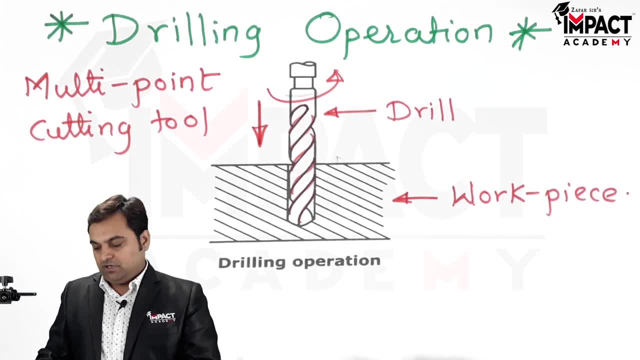 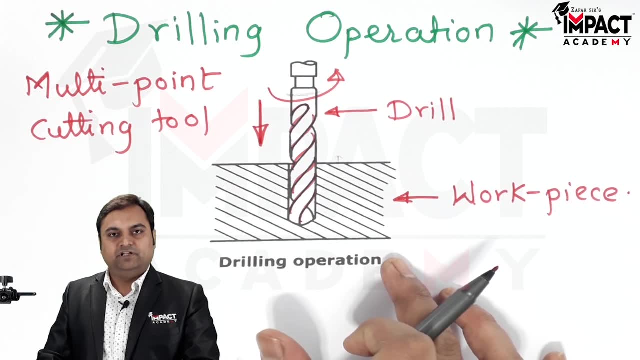 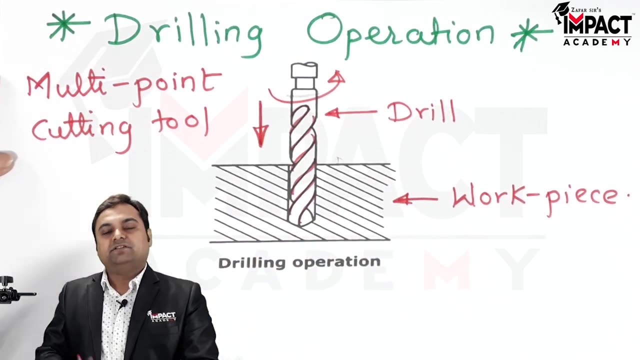 or the various kinds of drilling machines. But if we want to perform drilling operation on a lathe machine, in that case the workpiece is held in the chuck of the lathe machine, The workpiece is rotated in an anti-clockwise direction and this drilling tool is kept in the 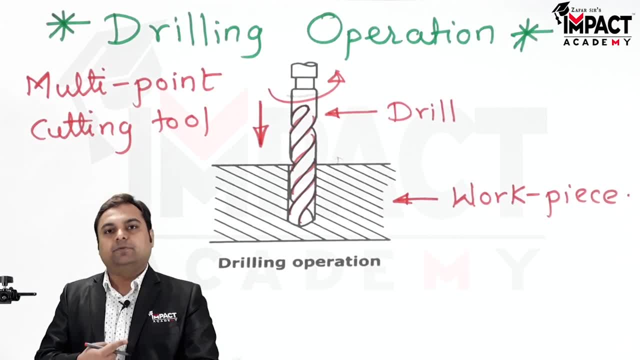 tail stock of the lathe machine and fed towards the workpiece. So in case of lathe machine, the workpiece also rotates. At the same time the rotation is also given to the drill. So both are rotating and the drill is fed into the workpiece and we are going to get the required hole. 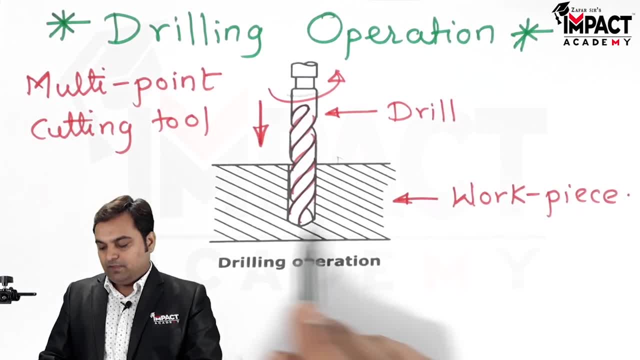 Whereas in case of portable drilling machines, the workpiece is stationary and the drill is fed inside the workpiece and at the same time it is rotated. Similarly, in case of all the drilling machines as well, the workpiece is kept stationary and the drill is rotated. 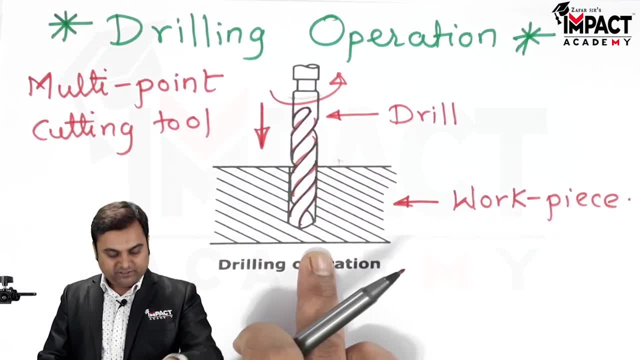 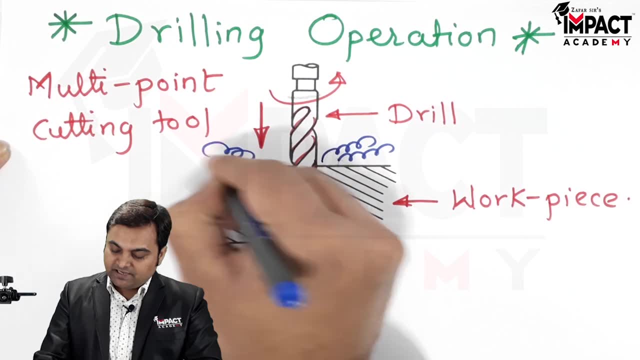 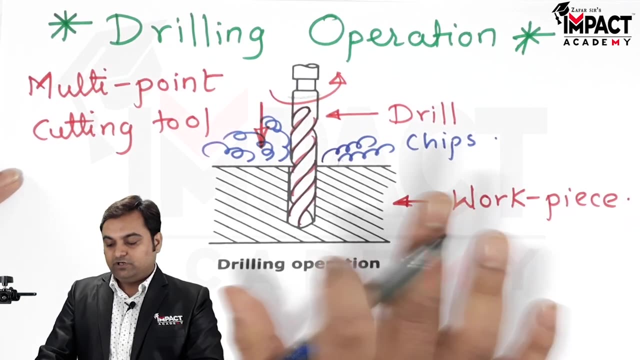 and fed into the workpiece to produce the required hole, and the material is removed from the workpiece in the form of small small chips, as I am showing it over here. It is removed in the form of small small chips and this is one of the primary machining operations. 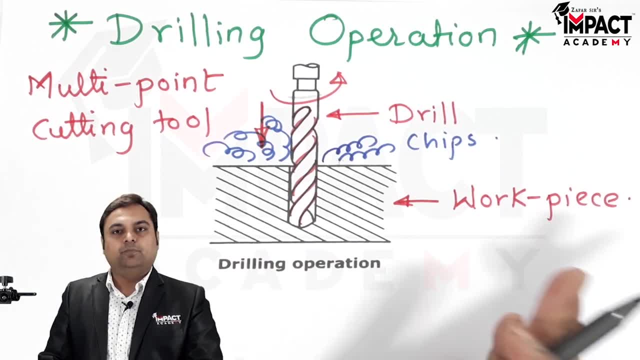 which is performed After drilling, we can go for the remaining operations. that is, either we can have boring, reaming, tapping or any other given operation. So this is one of the primary hole generating operations. So, in short, that was an explanation regarding the drilling operation. 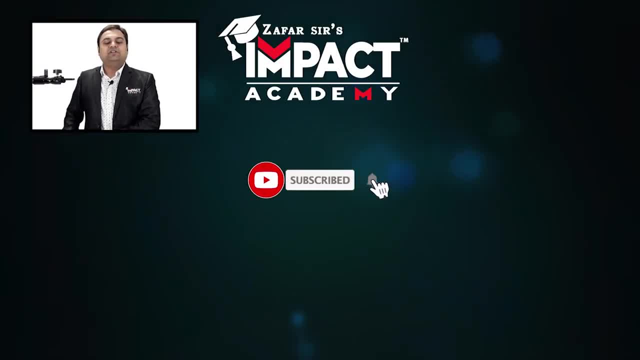 At the end. if you'll find my videos helpful, you can like, share, comment and subscribe our channel And share it amongst your family and friends. Thanks for watching.